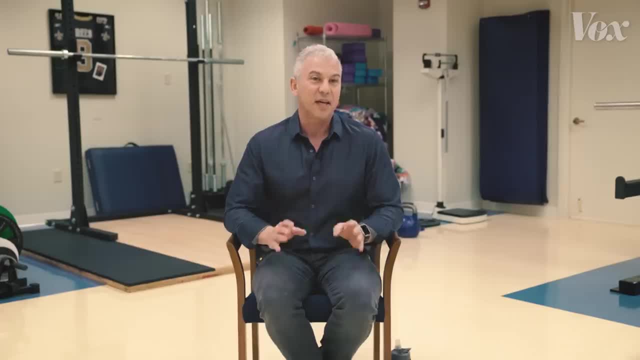 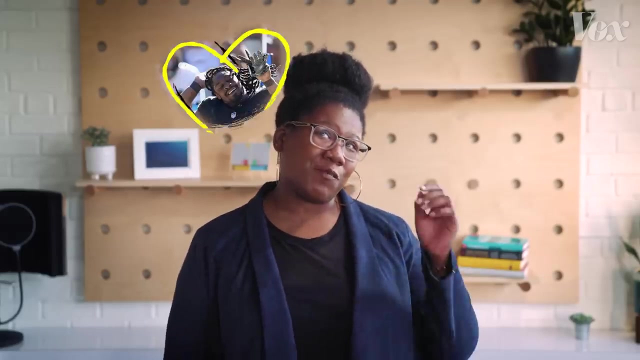 can separate being overweight from being obese. The major problem with using BMI as a marker of health when it comes to body weight, because it penalizes you if you have a lot of muscle and you're healthier. Let's use professional athlete Marshawn Lynch as an example. 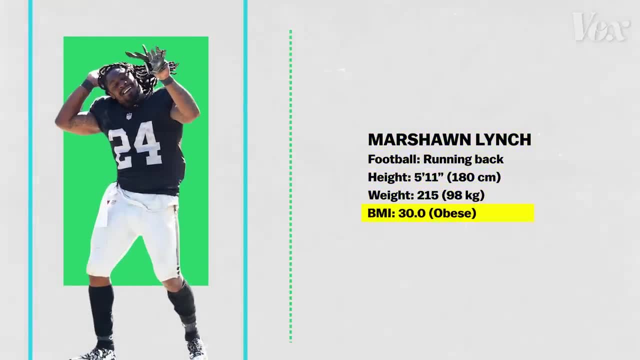 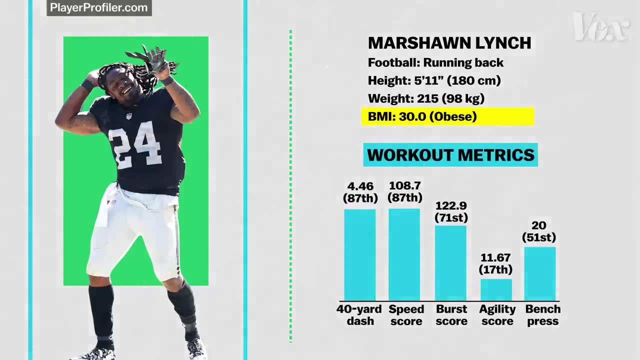 He's 5'11", 215 pounds, and his BMI is 30. He'd be categorized as obese. That's because BMI doesn't distinguish muscle from fat. Here we're really concentrating on how much muscle does somebody have, Because muscle is the metabolic engine. 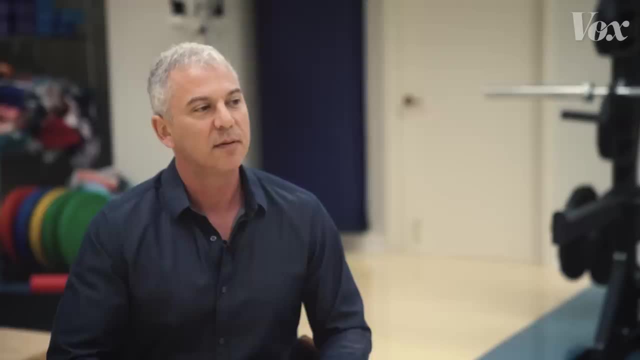 It's the thing that burns calories, And the more muscle you have, the easier it is for you to stay at a a lower, more healthy body fat percentage, not necessarily a BMI. In this way, BMI's reliability as an indicator of health. 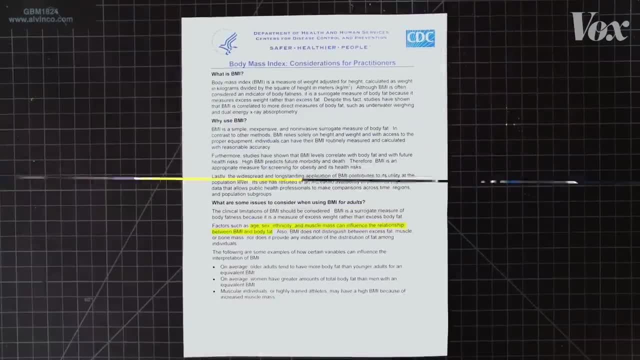 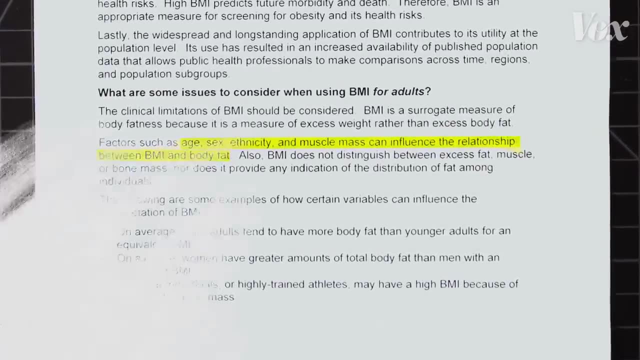 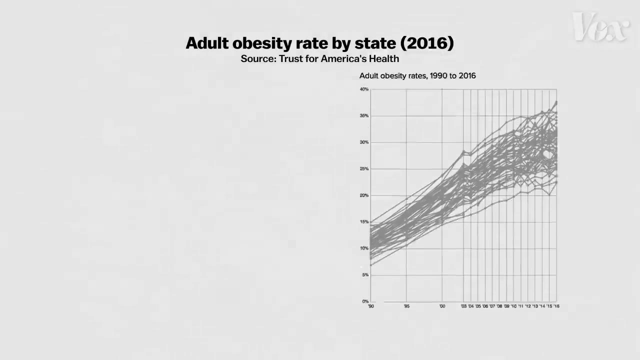 breaks down for athletes like Lynch. There are several more variables that can influence the interpretation of BMI, Things like age, gender and ethnicity. While BMI is a useful measure for a large population study, for example to compare relative obesity rates from state to state, it becomes more problematic. 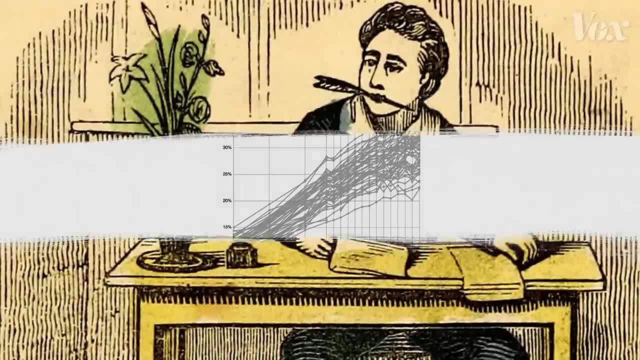 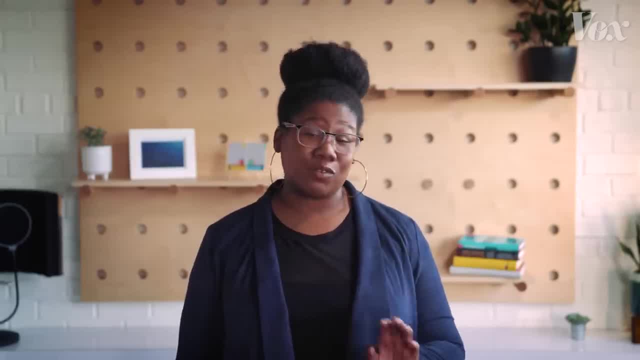 when you use it to determine an individual's health. The body mass index was introduced in the early 19th century. This guy who created the formula- I am so sorry I'm going to butcher his name- Lambert Adolphe Jacques Kutley. 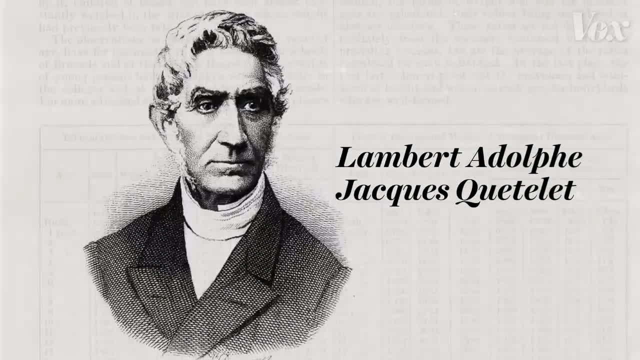 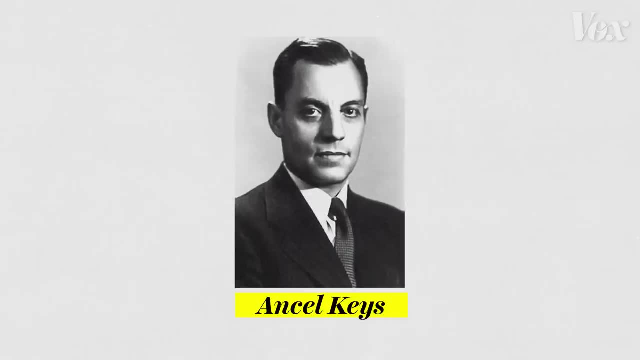 Wasn't even a physician. Kutley Was a Belgian mathematician. His reason for creating the formula was to study the normal man, not obesity. Its use shifted to study obesity because of Ansel Keys In 1972, Keys used the formula in his indices. 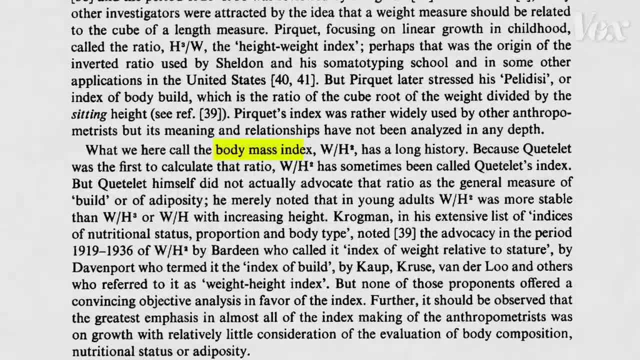 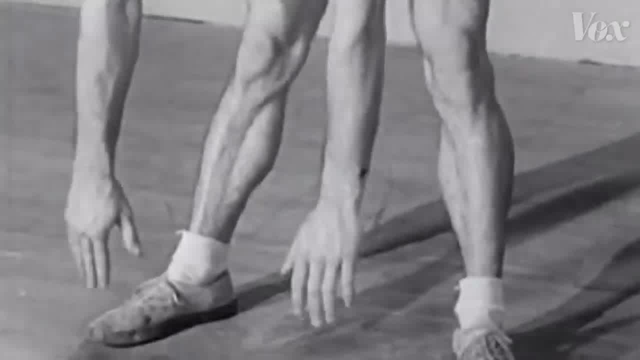 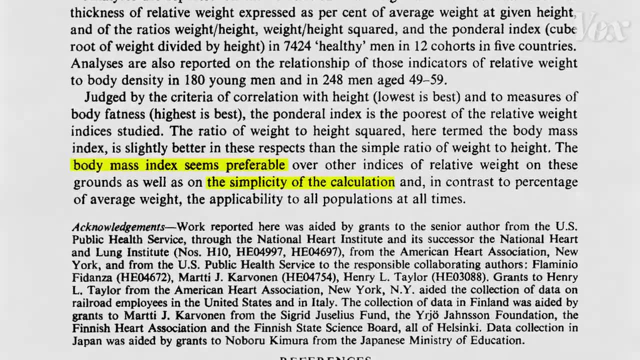 of relative weight and obesity study, renamed the formula to body mass index And from there the new measure caught on among researchers. Over the years its use in the health professional field grew and it's pretty much stuck around, since It's easy to use, cheap, fast and it's right about 80%. 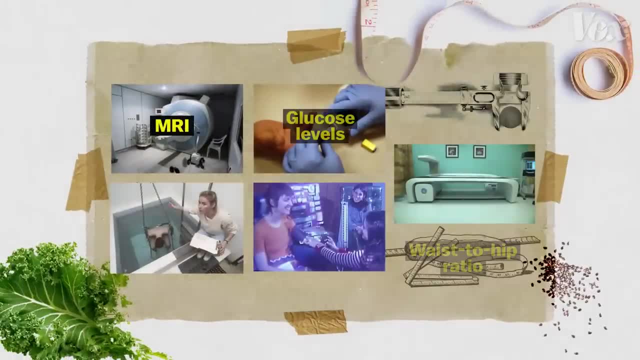 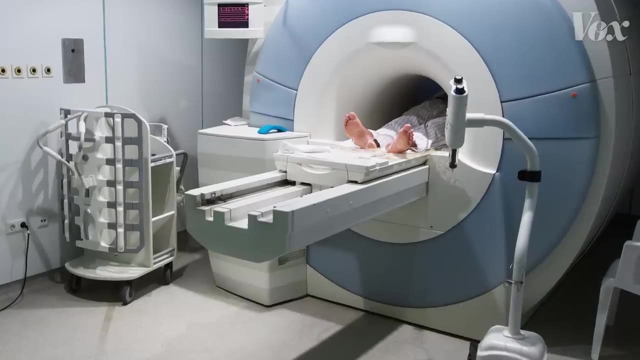 of the time. So even though BMI has stuck around for more than 200 years, it's not the be-all and end-all health indicator. There are more effective ways to assess body composition and overall health. Hydrostatic weighing or underwater weighing is an option, along with MRI scans.